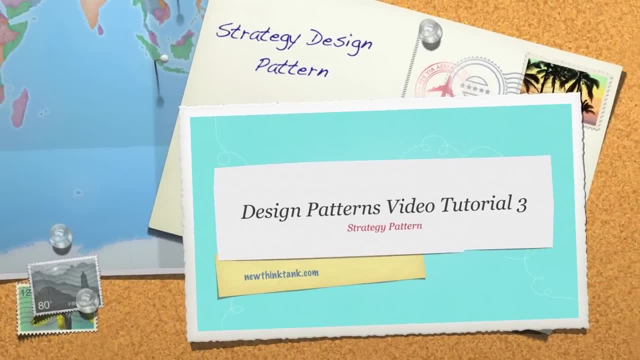 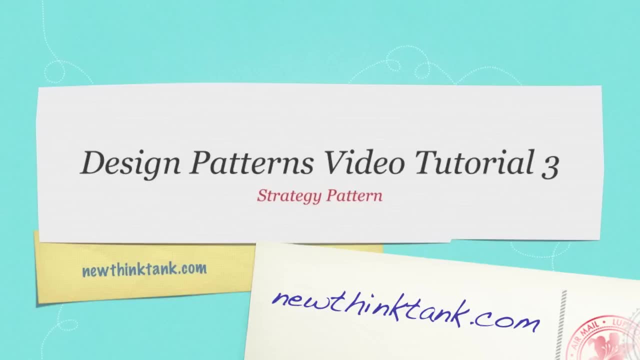 Well, hello internet and welcome to part three of my design patterns video tutorial. Today I'm going to do something a little bit different with this tutorial. This should be self-contained 100% just on the strategy pattern, unless you do not understand basic OOP concepts. If that's true, refer to part one and two of these tutorials. But from this point on, all of these tutorials will be 100% self-contained. And to teach you the strategy pattern, I'm going to write bad code so you can see in what situations you would need the strategy pattern. I'm also going to 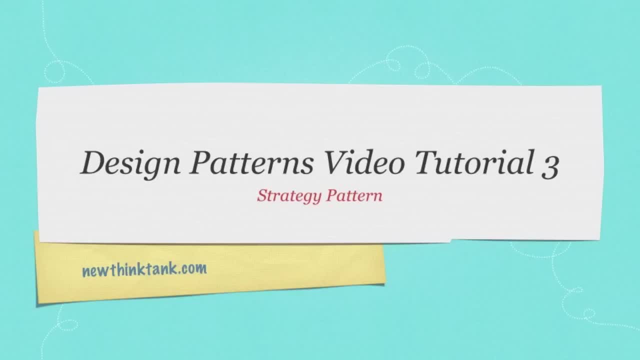 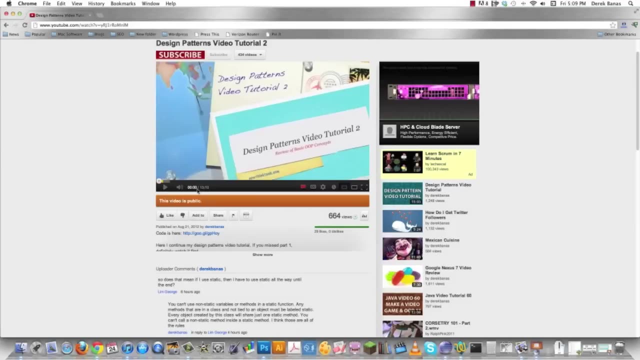 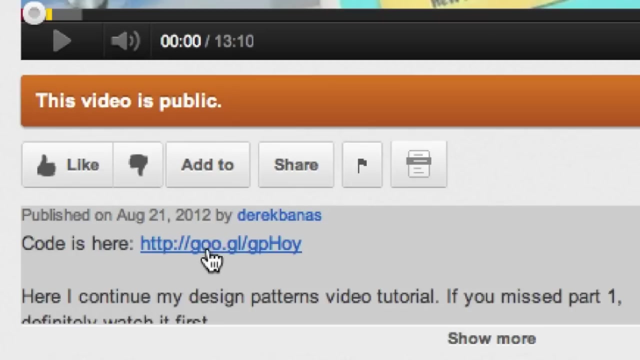 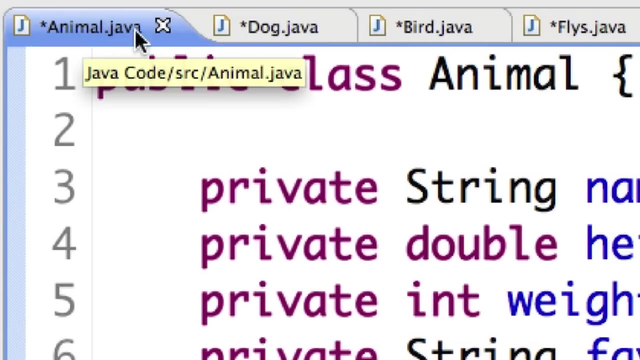 demonstrate it in code format, just like always, And then I'm also going to explain it using a presentation as well as a UML diagram. And, like always, all of the code is heavily commented, and this is another great way to learn this concept. Download the code and read the comments. It's free, so why not? So let's get into it, Okay, so here I am. over here, We have a couple classes to find. We have animaljava, and then we have two subclasses underneath of it: Dogjava and birdjava. 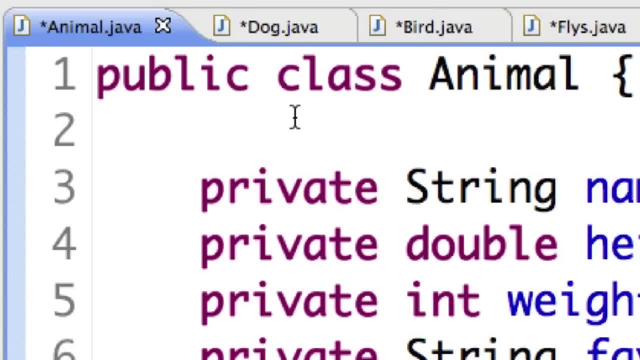 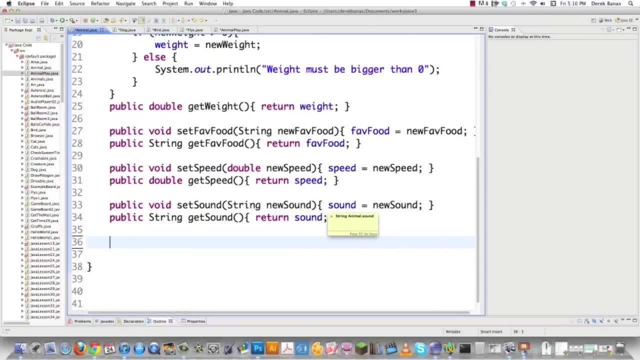 And what we're going to try to do here is figure out how we can give birdjava and other animals that are subclasses of animaljava the capability to fly. Now this is where the bad code part comes in, because I'm going to come in here and just think about how we could accomplish this using techniques that we've already learned. Well, one thing I could do is just come in here and go public void, fly and create a method inside of animaljava and then have it do some 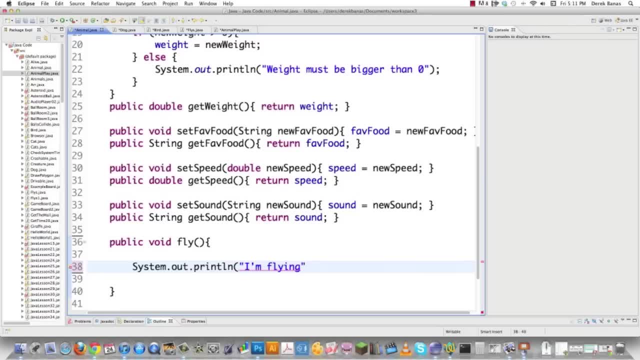 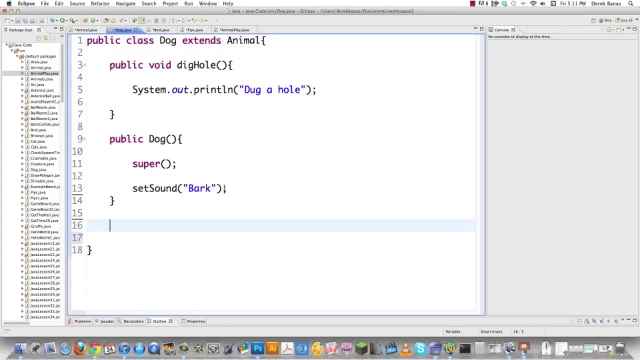 something like I am flying. Print that out on the screen And there you go. Well, why is this bad? Well, you never want to add any methods to a superclass like animaljava if they do not pertain to any subclasses. You need to separate what is different between subclasses and their superclass. But your answer to that might be like: oh, you're being silly because inside of dog I can just simply come in here and override, just like we've always done in the past, and just create my own. 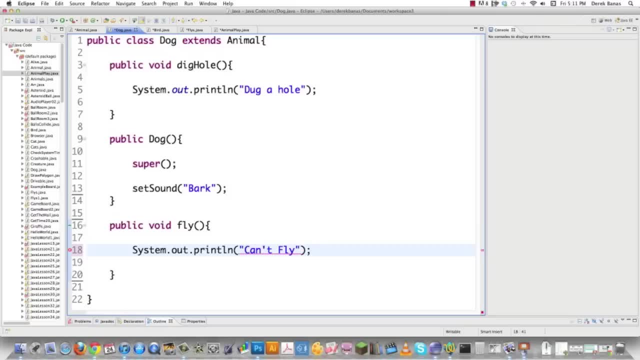 fly method and everything is going to be dandy And you could do that. but again, we're learning rules here on how to write good code. We need to continue to abstract out what is different and put just those things that are different inside of the classes. However, that would not make sense to come in there and just put it in the birdjava class because in that situation- because we would be creating a lot of duplicate code if we expect a lot of our animals to be able to fly. 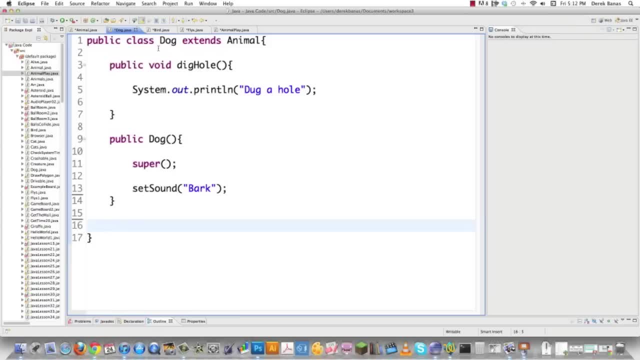 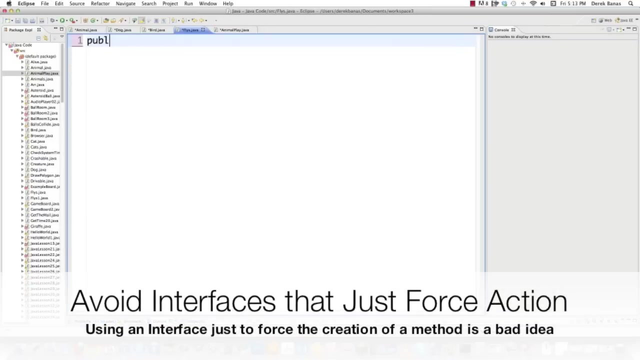 So we would go in there and continuously. every time we created a new animal and it just so happened to fly, we would go in and add in the method fly, over and over and over again. So we also want to avoid that issue. Let's go back over here and let's delete this, because that's just wrong. Don't want that. And you're also going to find, if you would come in here and create an interface, let's say called flies, that would then force all animals to figure out exactly how they're going to use the fly method, That is also going to 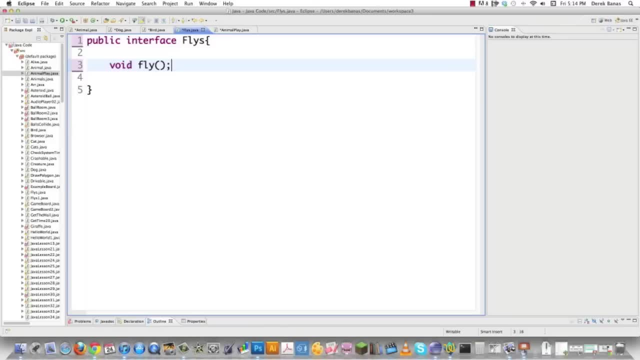 create a massive amount of duplicate code. Two basic principles that you really have to get into your head is: you want to always eliminate duplicate code, and you also want to eliminate any techniques that cause one class to affect others. A superclass change shouldn't break code in a subclass, and vice versa. If there is a situation in which that seems to be happening, you definitely want to rectify that. However, using the strategy pattern, we are going to use an interface, but we're going to use it in a completely different way In this situation. 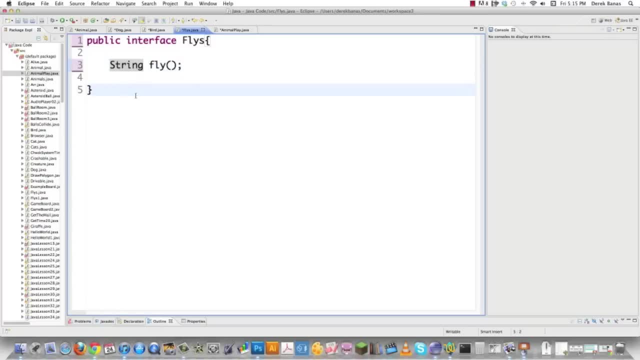 I'm going to create this interface flies, just like we did before, except in this situation it's going to return a string. That's not really important, so don't really focus on that. What is important is we are going to create separate classes. It flies, which is going to implement the flies interface, and then in this situation, because it's going to implement that, we're going to go add unimplemented methods and get rid of all this extra nonsense we don't need. And then, in this situation, we're going to go into return and I'm going to type something like this: 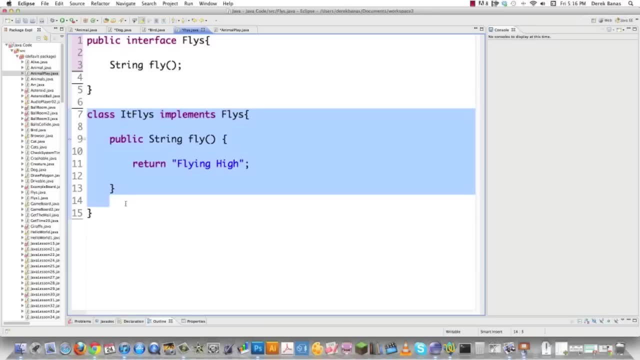 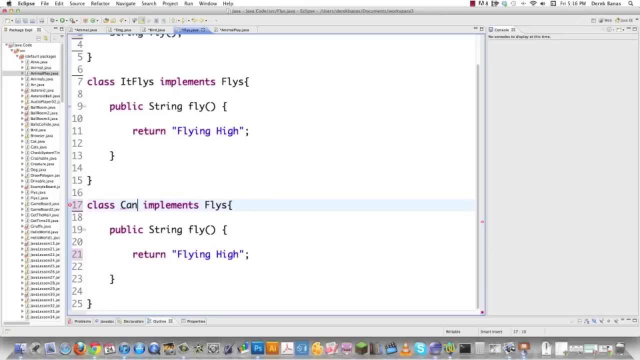 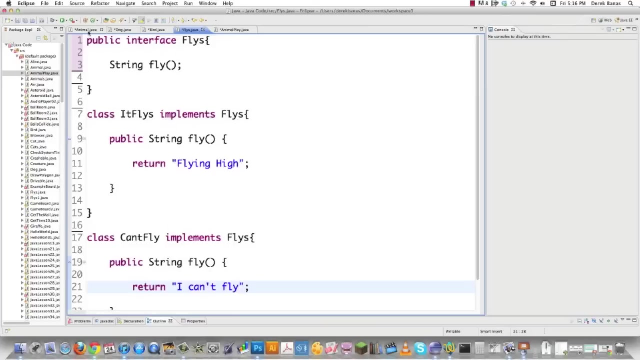 Something like flying high. And then I'm going to create another class, so I'm just going to copy this and it is also going to implement the flies interface, except it's going to be called can't fly. Yes, I know that's spelled incorrectly. And then here we're just going to change this to return I can't fly. And there you go. So now what we did was we created an interface and we're then going to use this interface inside of animal as an instance variable, and then we're going to dynamically change. 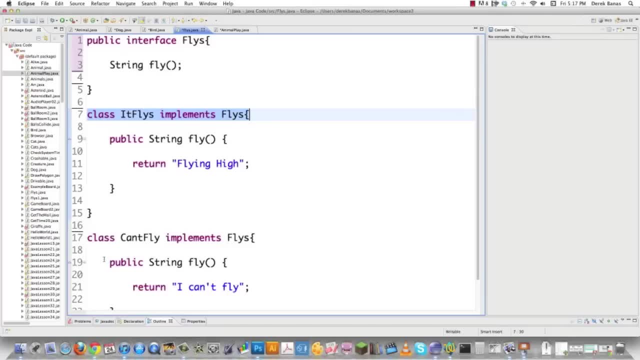 that instance variable to be either of type, class it flies or class can't fly, And why this is a great idea is the interface is implemented by many other different subclasses, and what this is going to allow us to do is create many different types of flying without affecting animal or any of the subclasses, And then, from that point on, classes that implement this new fly interface are going to allow those classes to use that code, while also eliminating code duplication. 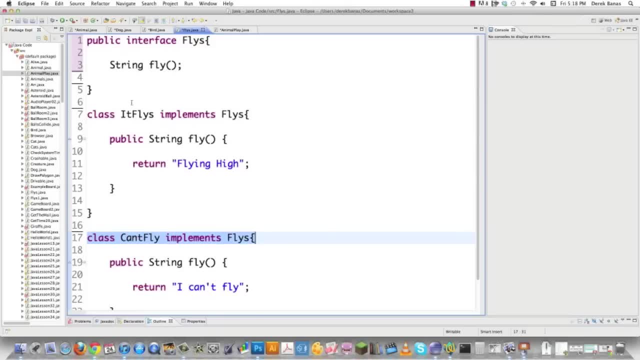 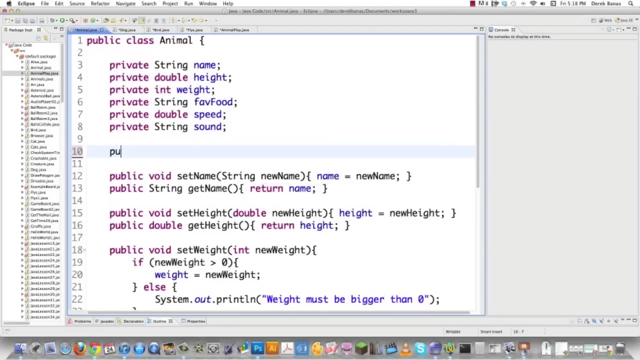 And this is known- this is a technical term- as decoupling, which means that we are encapsulating the concept or the behavior that varies, and that behavior or concept is the capability to fly. If you're not quite getting everything, don't worry about it. I'm going to show the two in multiple different ways. So let's jump over into animal and implement this, And it's going to be quite easy to implement. Remember, we're just going to create a new instance variable. I'm going to make it public, I'm going to call it flies and it's going to be of type flies. 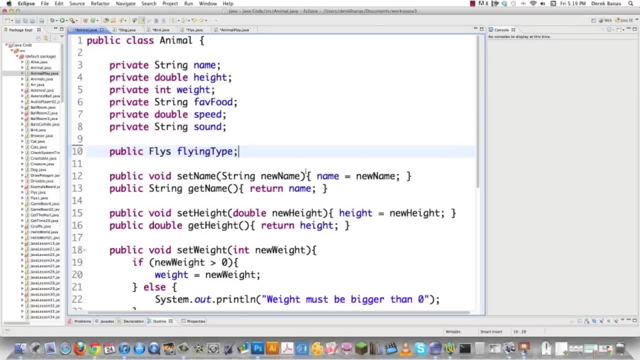 And I'm just going to go flying type like that. So instead of using an interface in a traditional way, we use instance variable. that is a subclass of the flies interface. An animal doesn't care what flying type does, it just knows the behavior is available to all of its subclasses, And this is also known as composition. Instead of inheriting an ability through inheritance, the class is composed with objects with the right ability built in. And another great thing about composition is it allows you to change the capability. 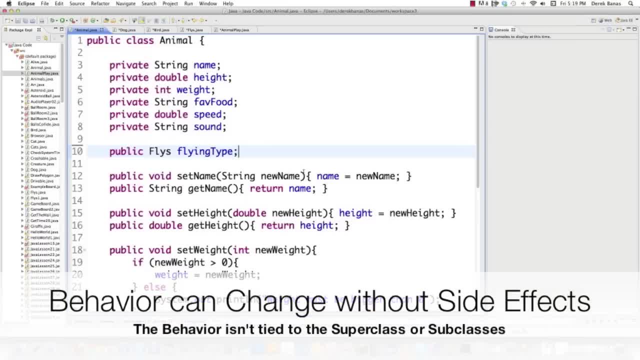 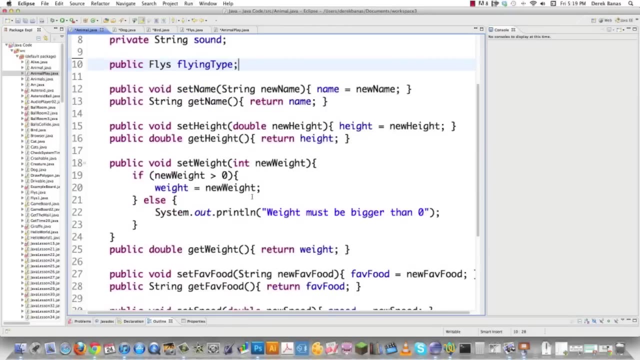 of objects at runtime. So if you create an object, an animal object, and it starts off as a non-flying object, but then it grows a set of wings and all of a sudden can fly dynamically, you can go in and say: okay, I know, this object didn't fly before, but now it does. So it gives you a never ending supply of different capabilities. 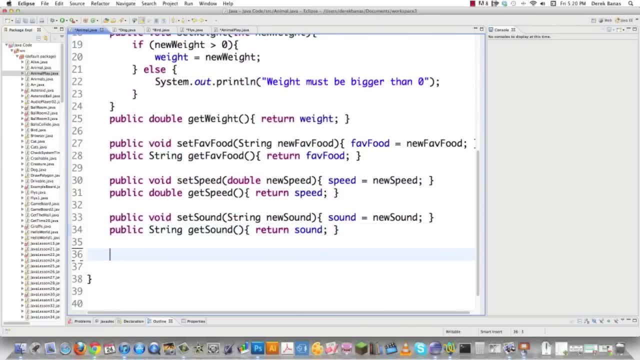 So now that we've created this guy, we're going to be able to just zoom down inside of animaljava and type in public string: try to fly, Right like this, and then it's going to return flying type and it's going to call the fly method: right like that. and 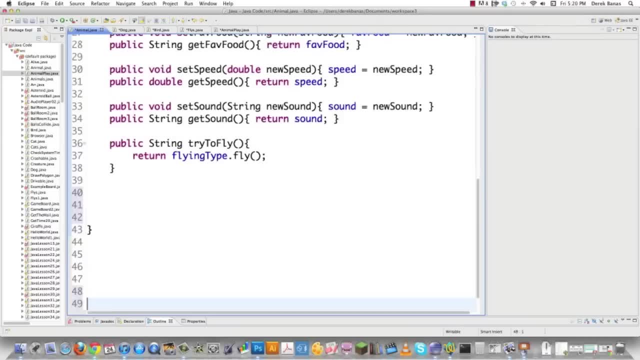 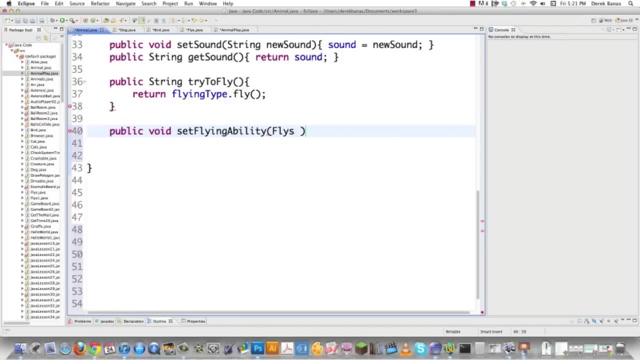 then another thing: we're going to make this all dynamic, which of course we want to if possible. we're going to go public void, set flying ability and it's going to be passed a flies object which is going to be new fly type, and then we can set flying type dynamically, new fly type by setting. 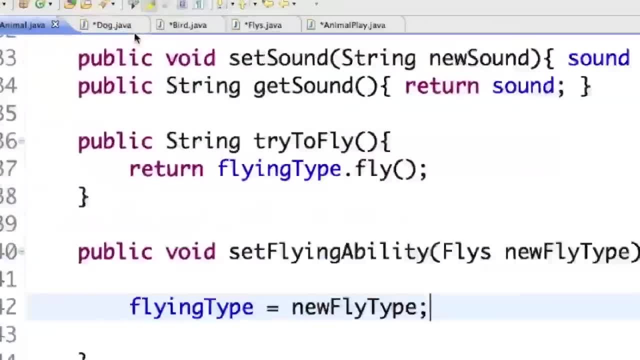 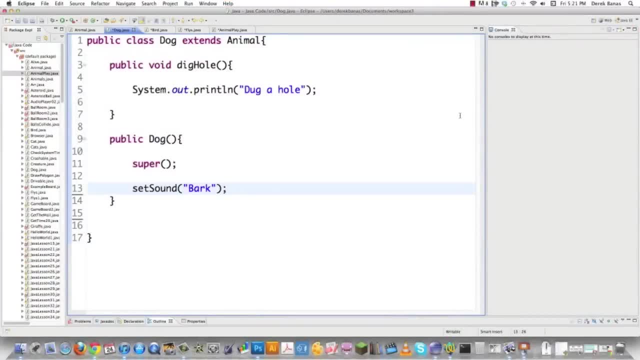 it to that object. so let's save that. so now, what are we going to have to do with dogjava and birdjava to make those work? actually very little. I'm just going to go into the constructor area whenever our dog object is built and we're going to say flying type is equal to new and in this situation we're. 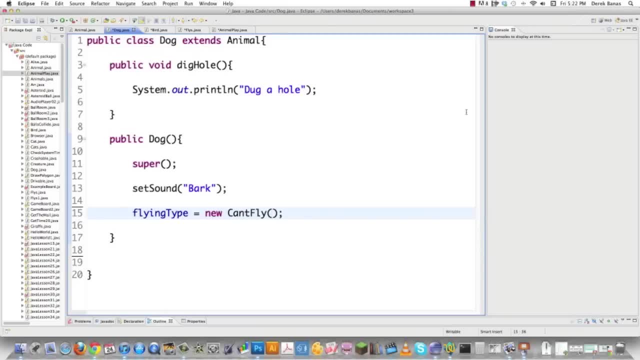 going to call: can't fly. this is going to set the fly interface polymorphically, and this is also, of course, going to set it as a non-flying animal. and by polymorphically, of course, I just mean we're going to set it as a non-flying animal, and by polymorphically we're going to set it as a non-flying. 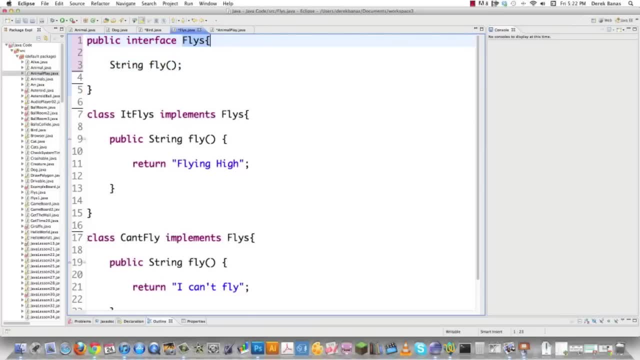 animal and we're going to refer to the flies interface, but we're going to set it to use can't fly, the can't fly class, underneath of interface. so that's it. that's all we need to do with dog to give it the capability to not fly. and you might say to yourself, well, the bird must be really hard to get. 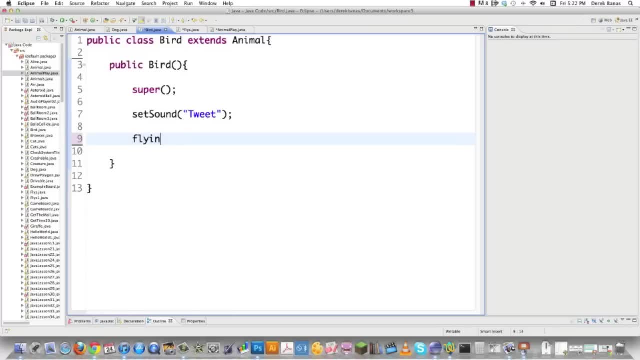 it to fly, of course, nope, just going to go in and go flying type is equal to new. it flies. so we're using polymorphism, we're doing all kinds of crazy stuff and that's it. you're done. so now let me try this tricked out. 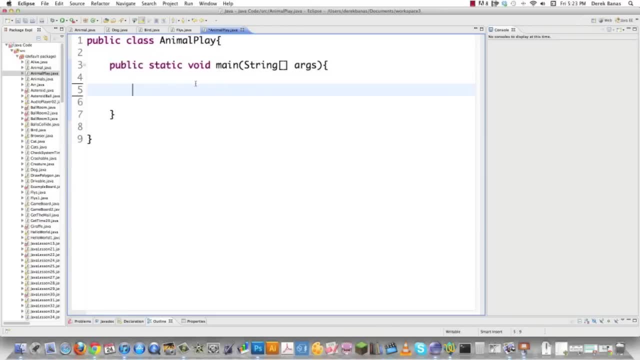 program. let's just file, save that, and we're going to jump into animal play dot java. we're just going to create some things. so I'm going to create an animal called sparky, and he's going to be a dog. and then I'm going to create another animal called tweety, and she's going to be a bird, and then go. 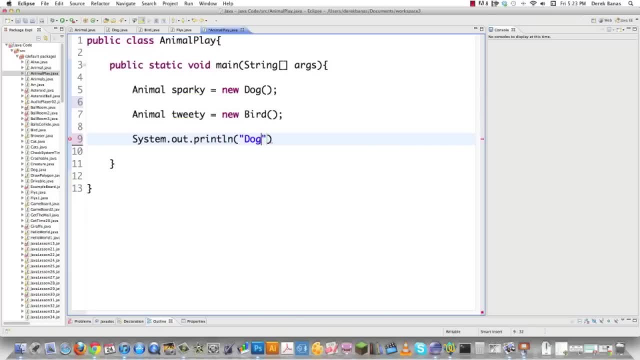 system out print line. and let's say we go dog and then have sparky, figure out if he can fly or not, and see what it's printing out on the screen. and then we're going to do the same exact thing with tweety, but we're just going to say: bird here, tweety file, save it, execute it, see what happens there. you can. 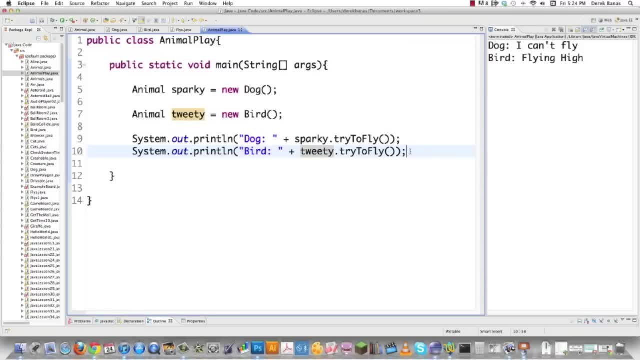 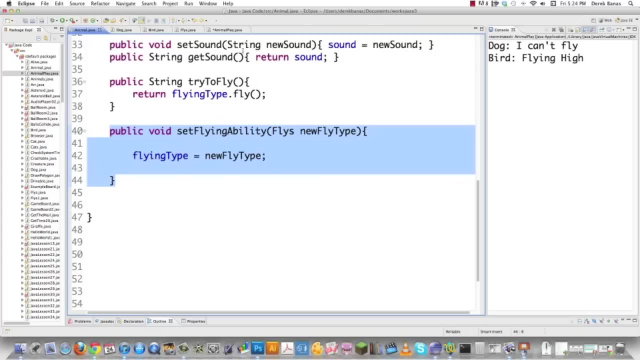 say: dog, I can't fly bird flying high, just the way we want it. and then I'm going to come over here. remember animal dot java. I created this method here that's going to allow me to dynamically set my flying ability. let's say, our dog here all of a sudden gets this amazing ability to fly. 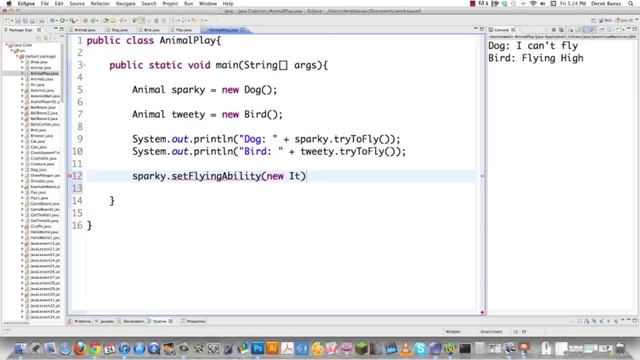 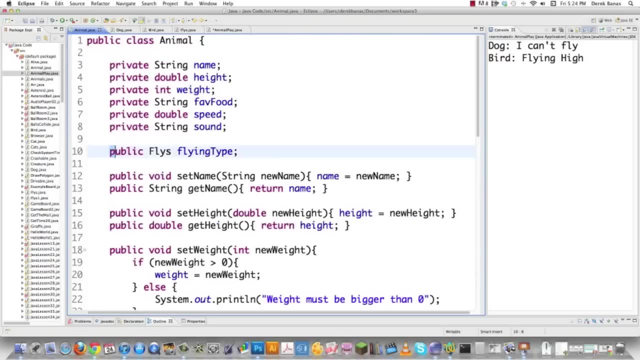 flying ability. I'm just going to create new object inside of the dog object by going in and setting the instance variable. and then I'm going to create a new object inside of the dog object by going in and setting the instance variable variable for animaljava. So all I'm doing is passing it a new one of these flying types. 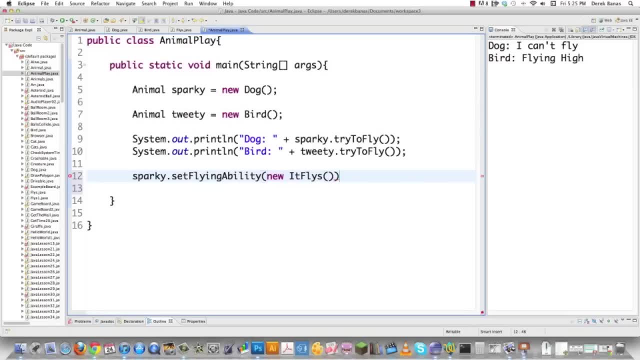 inside of here. And to do so, just go hit flies, Just create it File save. And now, after doing that, boom, File save, Proceed. And there you see, now the dog flies. So that's the code for it. Now I'm going to jump over and show you a UML diagram to sort of make 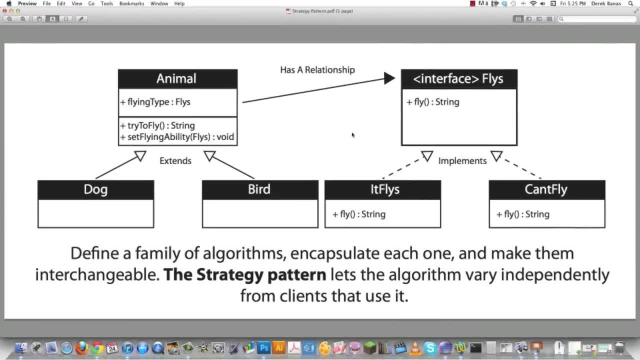 sure that I completely cement this in your head. Okay, so here is our UML diagram. Basically, we have our animal And the plus here means that this is a public instance, variable or a field And its name is flying type and it is of type flies And flies is the interface. 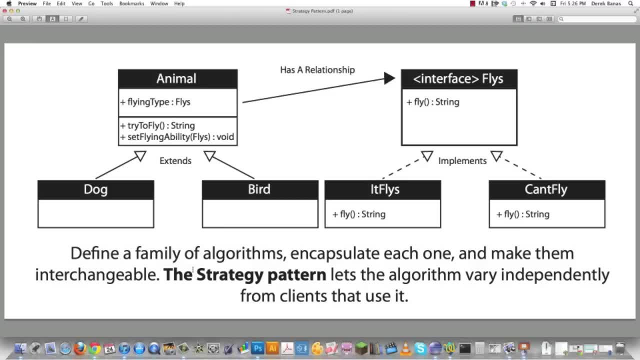 over here And the actual strategy involved in the strategy pattern is to define a family of algorithms. These are the algorithms. It flies or it can't fly There. they are just those two, Encapsulate each one and make them interchangeable. So we're going to encapsulate. 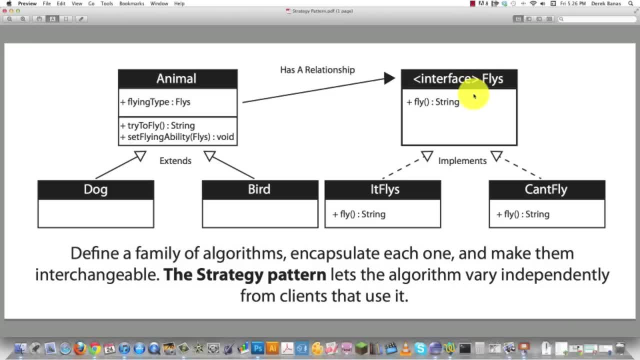 them inside of this interface called flies, And then we're going to encapsulate them inside of this interface called flies, And then we're going to encapsulate them inside of this interface called flies, And then we're going to allow the animal over here, as well as all of its 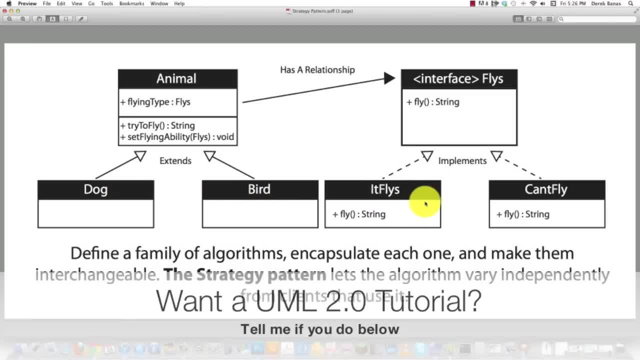 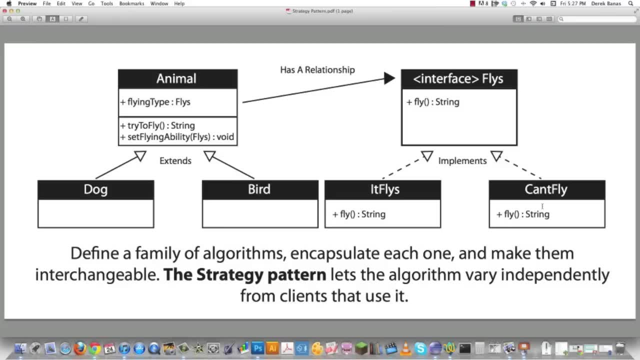 subclasses to dynamically switch between either being a it flies or a can't fly. What's great about the strategy pattern is it lets the algorithm vary independently from clients that use it, So it's really cool. All this different stuff is all inside of there, So 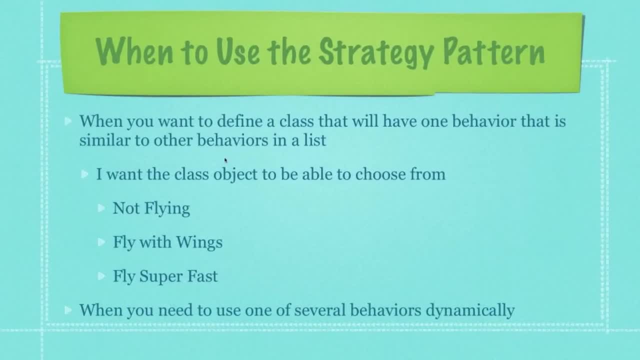 let's review. You are going to use the strategy pattern when you want to define a class that will have one behavior that is similar to all the other behaviors in a list. So let's say we have animals that fly and animals that don't fly. The similarity is that flying